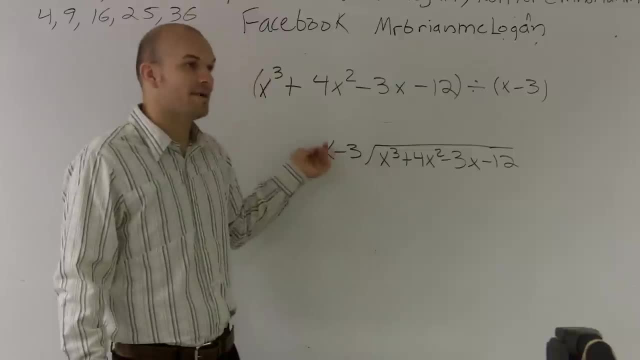 I can't divide my 3 into my X. However, I can divide my X into these X's, So I'm going to start with my first number, And that's the number I'm always going to work with as far as dividing. 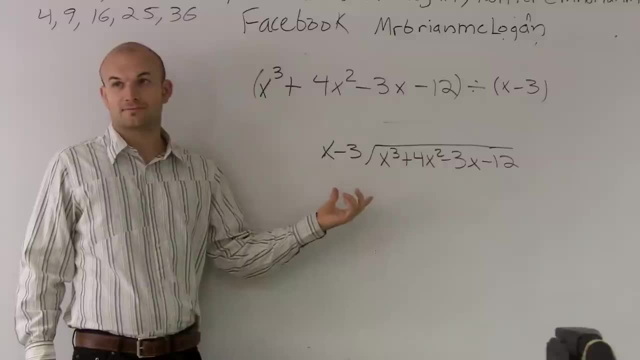 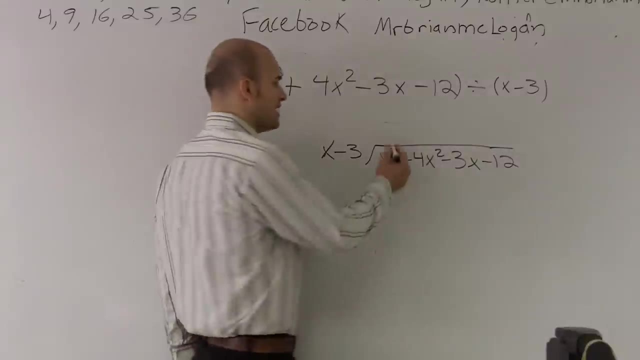 So if I can't divide this X into a number, it can't be divided, All right. So I look at this first. I say X, can that divide into X cubed? And yes, it can. It can go in there X squared times. 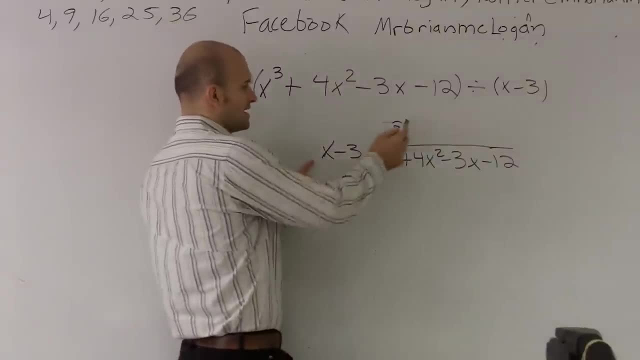 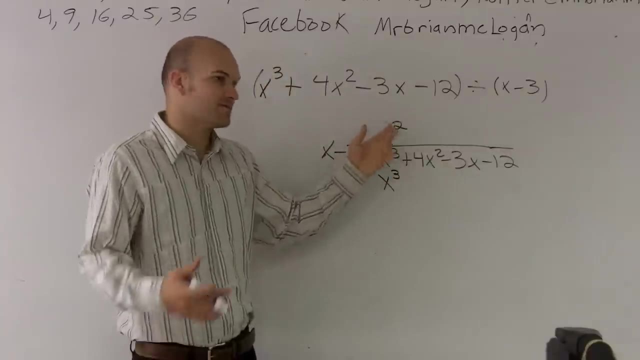 What do I mean? it goes in there X squared times. Well, you can check your work: X squared times, X gives you X cubed. Okay, So therefore I know it's yes, X cubed goes in there. X squared times, because those two multiplied give me X cubed. 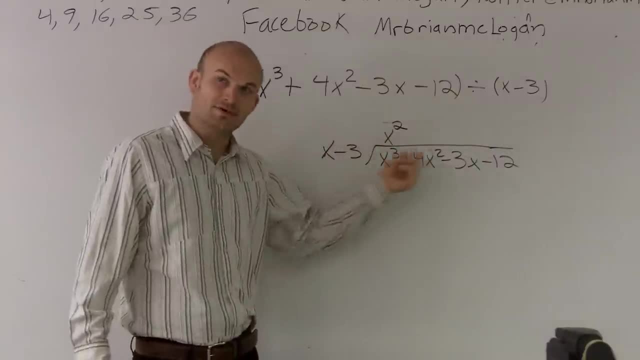 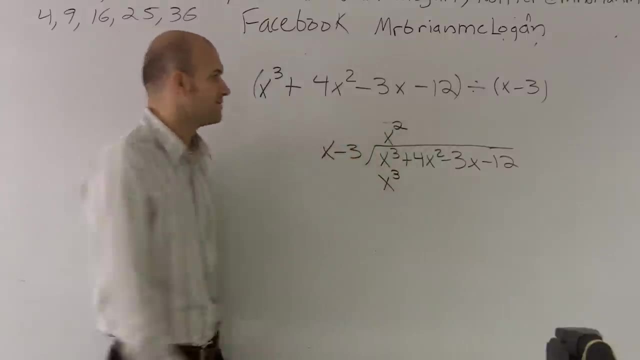 Now this is where we get our negative 3 back into the game. This is how we use this negative 3.. When I multiply back, I got to make sure I multiply the X squared also times my negative 3.. So X squared times negative 3 is a negative 3X squared. 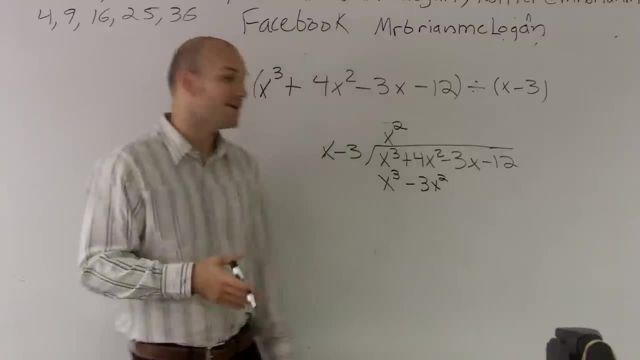 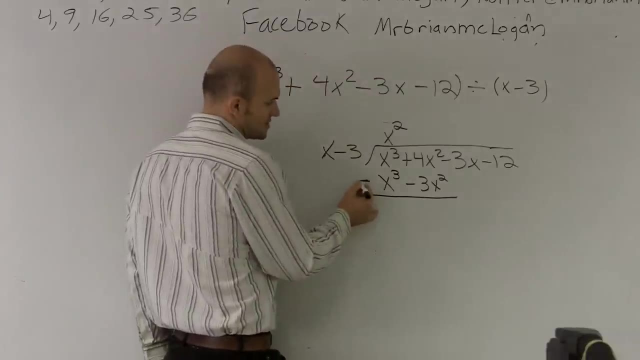 Do you guys want to know where everybody makes a mistake? Where, Right here? When you're done with that, we need to subtract the two lines, right, So everybody writes a subtraction sign And then you do X cubed minus X cubed is 0X cubed, which is 0. 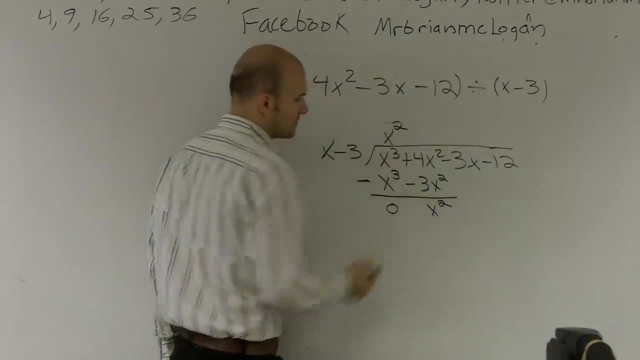 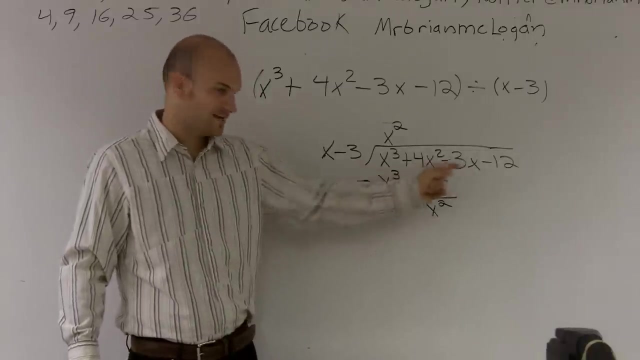 Then they do: 4X squared minus 3X is X squared, It's plus. Okay, It is plus, because what you need to notice is this is: I'm subtracting this whole line, So if you want to, you can think of this as like parentheses. 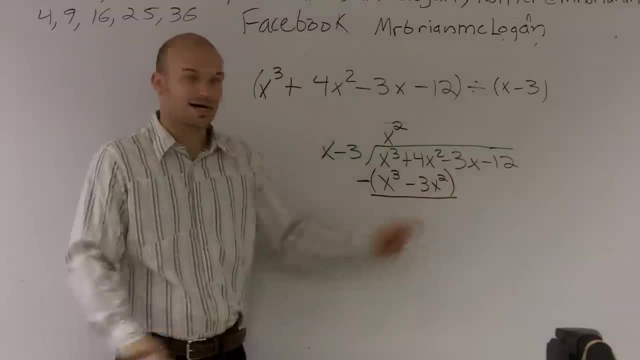 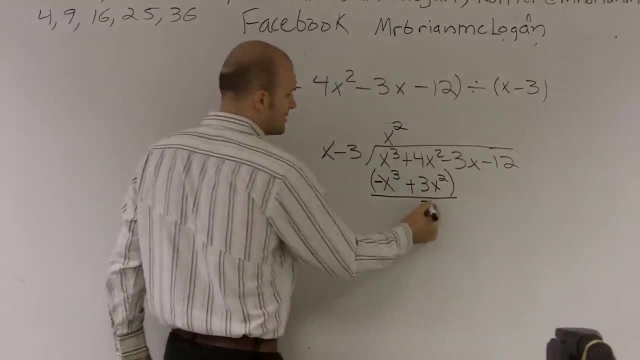 I'm subtracting everything that's on this line. So therefore that's a negative And that now becomes a positive. So it's really. your answer is going to be 7X squared. No, That make sense. No, Okay. 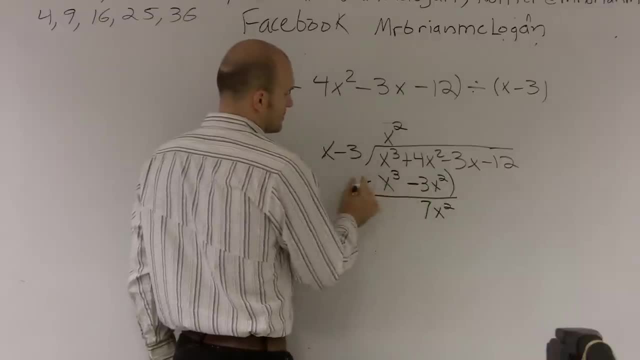 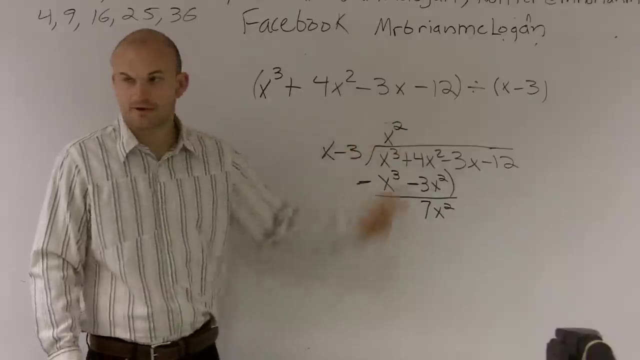 I mean, look at it this way: Wait till the answer is 7X squared below: Yes, All right, You're subtracting the whole line, right? That's a negative 3X. right X squared times negative 3X. 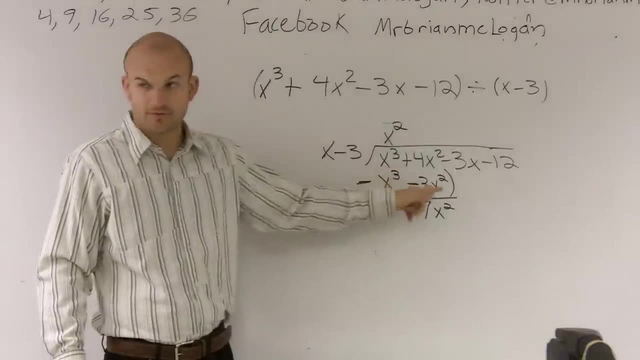 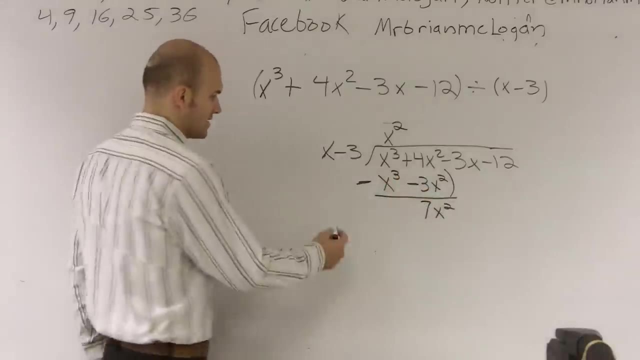 4X squared. 4X squared minus a negative 3X squared. Double negative makes it a what Positive? Positive. So that's where I get a 7X squared. Just think of it this way: It's 4 minus a negative 3X squared. 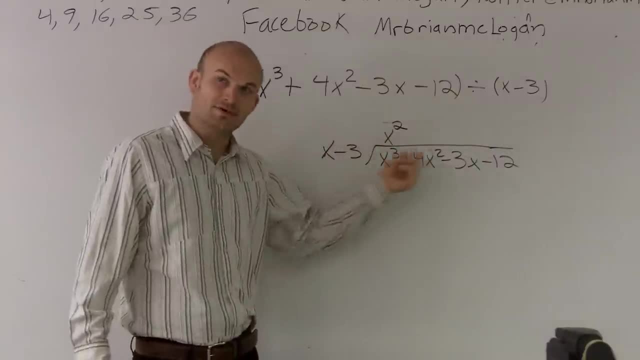 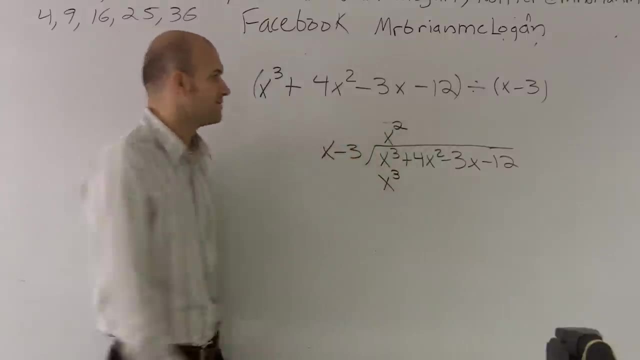 Now this is where we get our negative 3 back into the game. This is how we use this negative 3.. When I multiply back, I got to make sure I multiply the X squared also times my negative 3.. So X squared times negative 3 is a negative 3X squared. 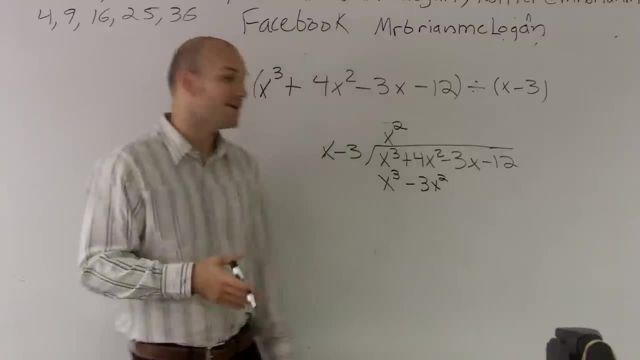 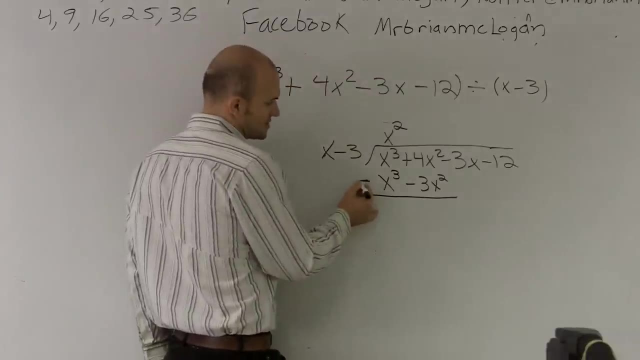 Do you guys want to know where everybody makes a mistake? Where, Right here? When you're done with that, we need to subtract the two lines, right, So everybody writes a subtraction sign And then you do X cubed minus X cubed is 0X cubed, which is 0. 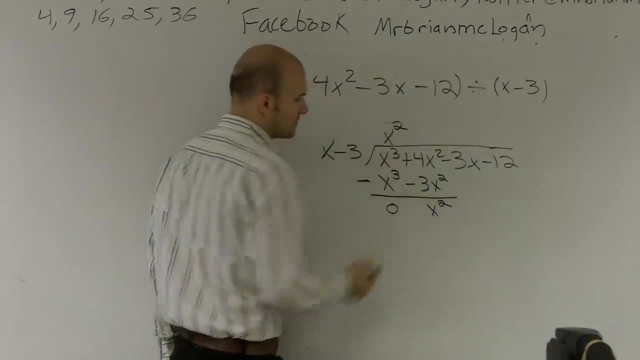 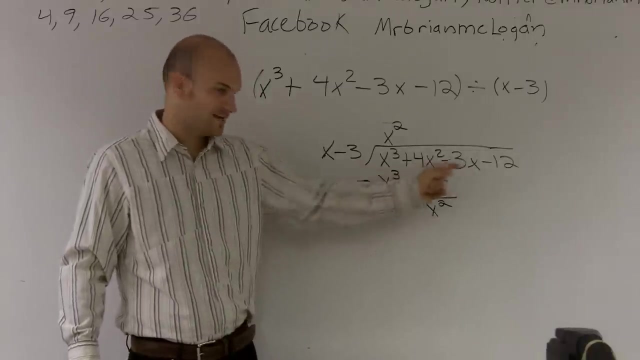 Then they do: 4X squared minus 3X is X squared, It's plus. Okay, It is plus, because what you need to notice is this is: I'm subtracting this whole line, So if you want to, you can think of this as like parentheses. 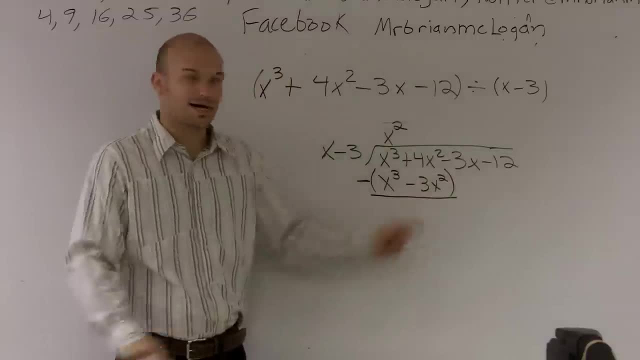 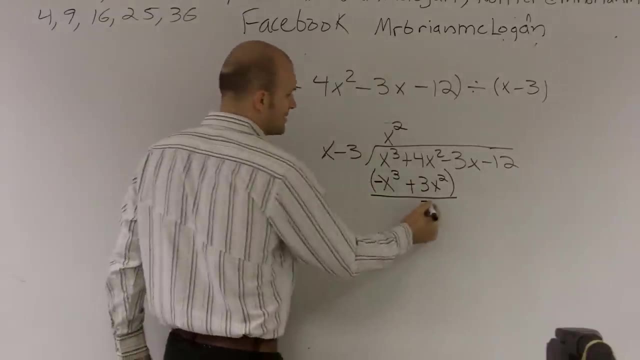 I'm subtracting everything that's on this line. So therefore that's a negative and that now becomes a positive. So it's really your answer is going to be 7X squared. No, That make sense. No, Okay, It doesn't make sense at all. 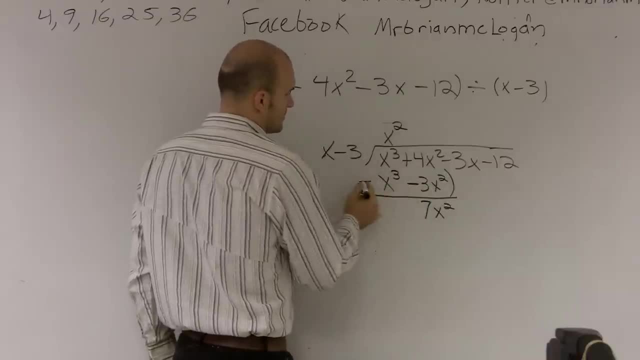 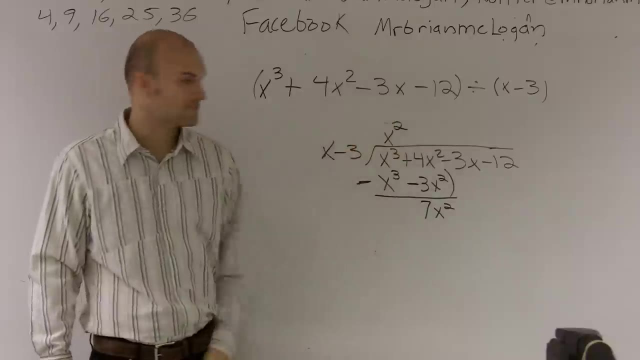 I mean, look at it this way, Wait till the answer is 7X squared below. Yes, All right. All right, You're subtracting the whole line, right? That's a negative 3X. right X squared times negative 3X. 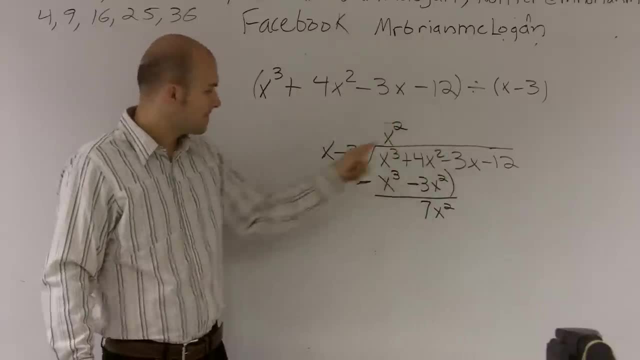 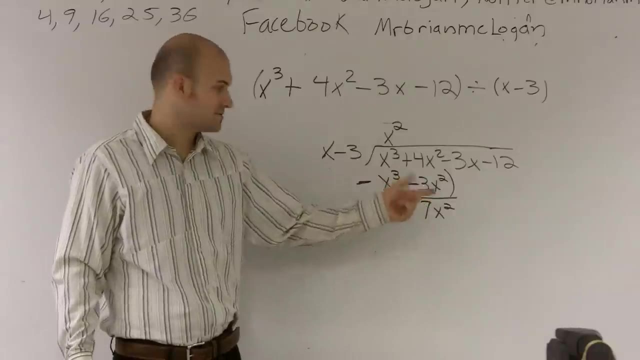 Okay, So 4X squared minus a negative 3X squared. Double negative makes it a what Positive? Positive. So that's where I get a 7X squared. Just think of it this way: It's 4 minus a negative 3X squared. 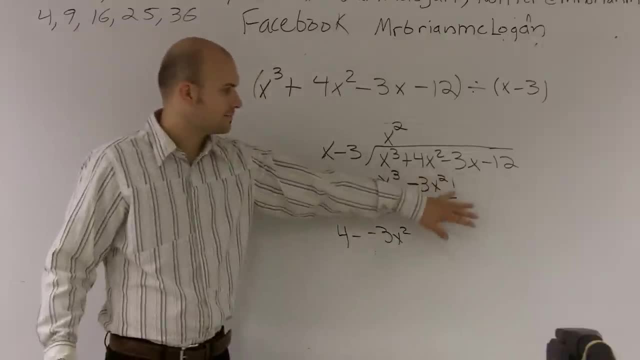 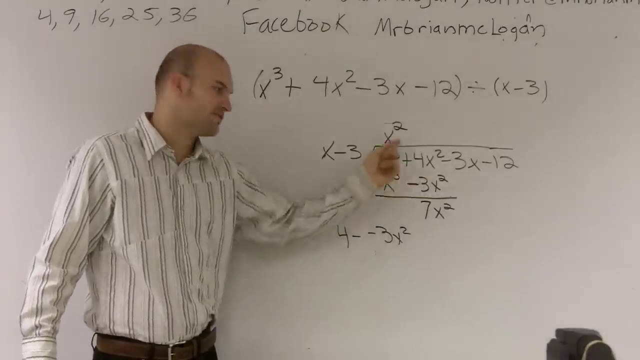 Oh, you confuse me when you put the parentheses in there. Right, Well, Just the okay, It's just normal. It's just 4 minus negative 3X. But so many students don't want to go back to this negative and they always forget it. 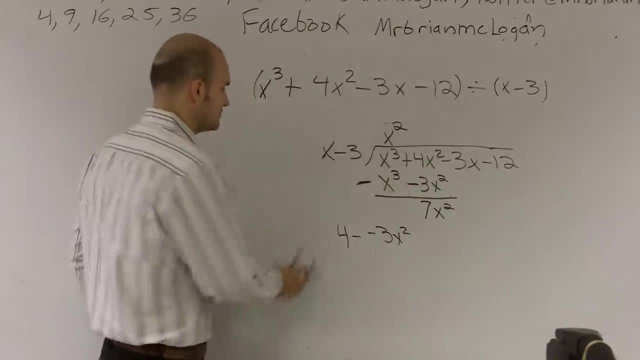 So they just do the whatever signs in front, They're just going to go back and forth, and they're just going to go back and forth. And so now I say, because X go into 7X squared, it goes in there 7X times. 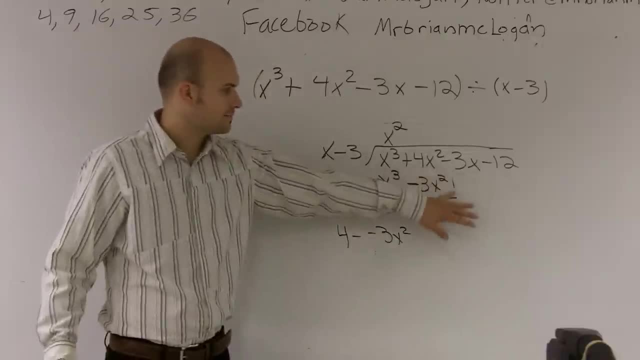 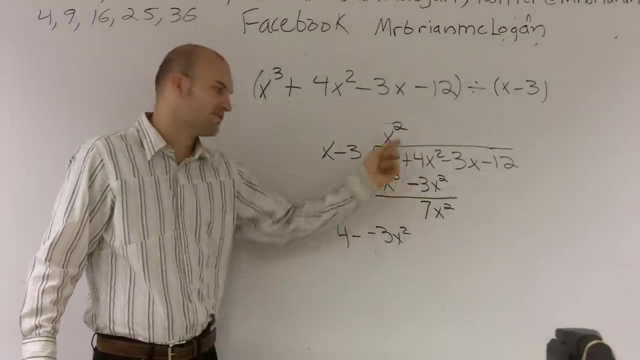 Oh, you confuse me when you put the parentheses in there. Right, Well, Just the okay, It's just normal. It's just 4 minus negative 3X. But so many students don't want to go back to this negative and they always forget it. 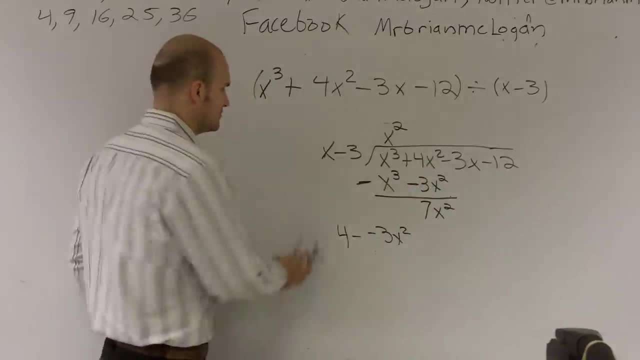 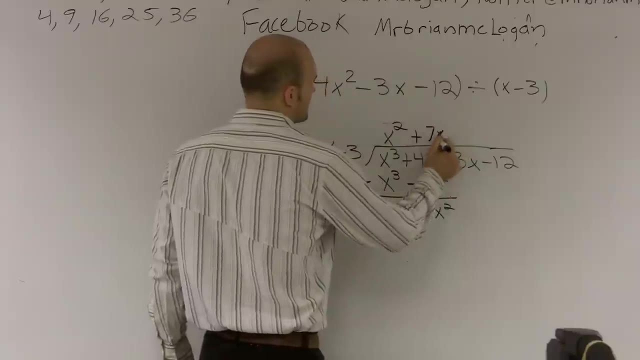 So they just do whatever sign's in front of there. And so now I say: because X, go into 7X squared, it goes in there 7X times. 7X times X is 7X squared, Easy. 7X times negative, 3 is a negative 21.. 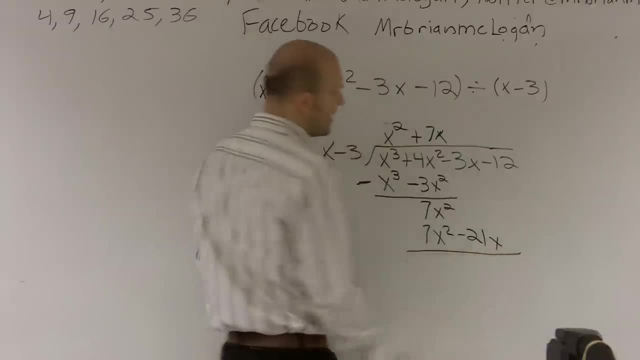 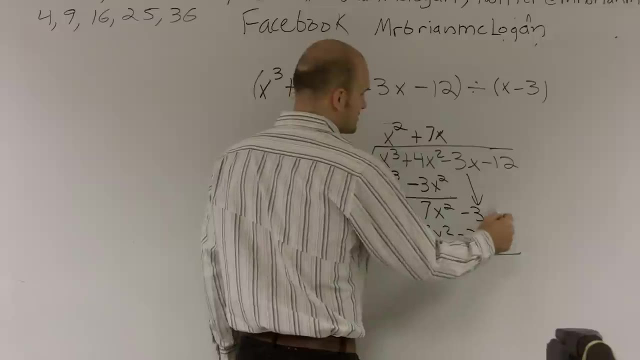 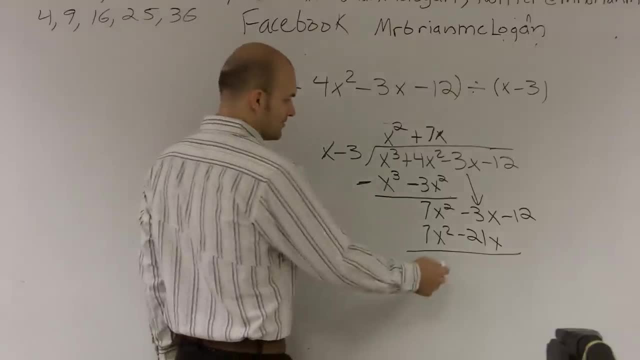 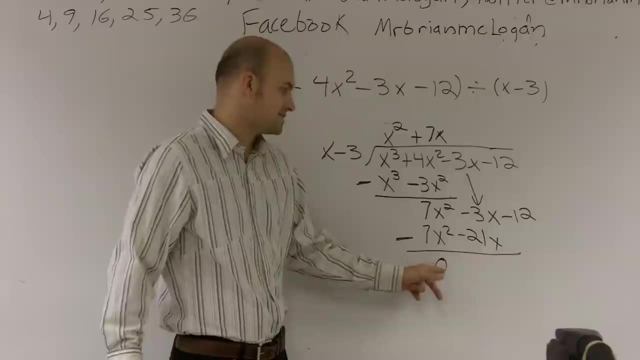 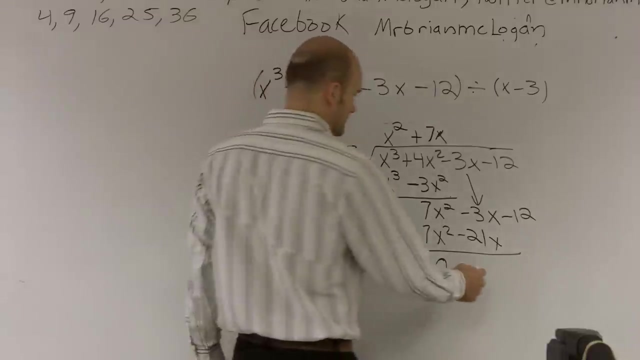 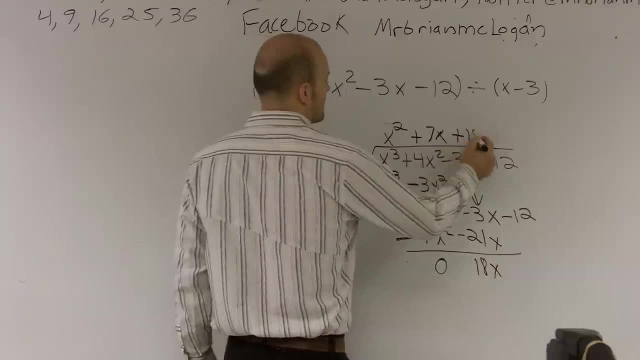 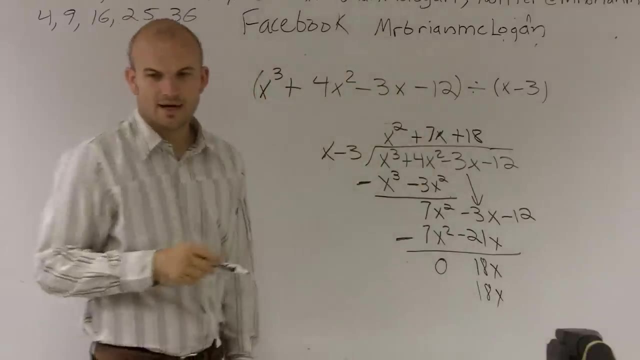 X goes into 18X 18 times. 18 times X is 18X. 18 times negative, 3 is a negative 54.. 18 times negative 3 is a negative 54.. Bring down my negative 12.. This gives me 40.. 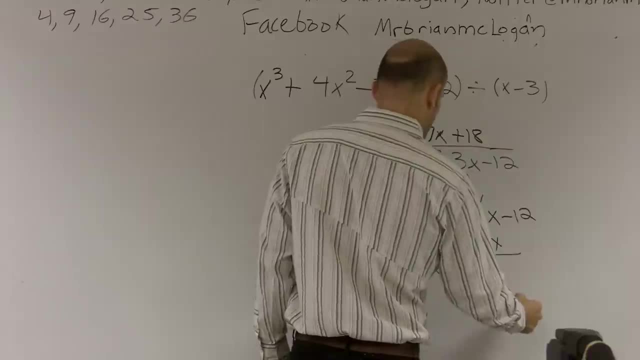 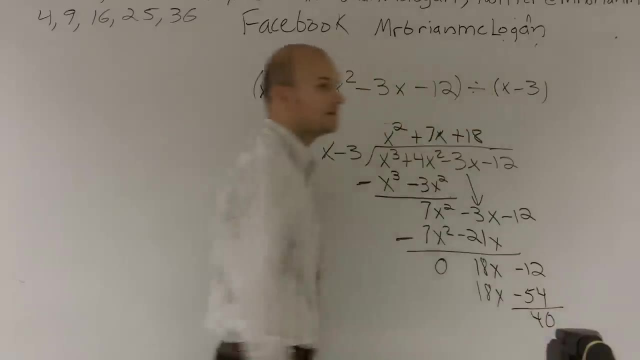 Negative 12 minus a negative 54 gives me 40. Now do you guys remember in what was it third or fourth grade? you guys did like R. It was like five, The main degree, All right. so remember, you did negative 4 and negative 3.. 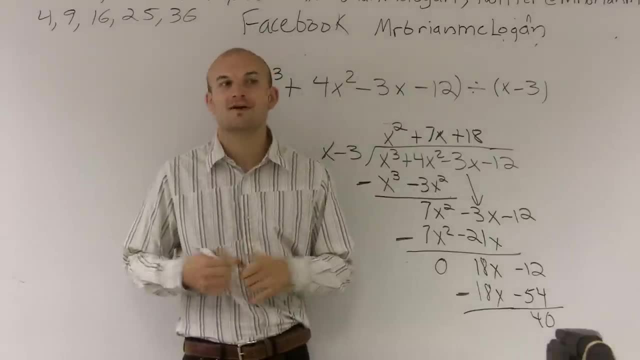 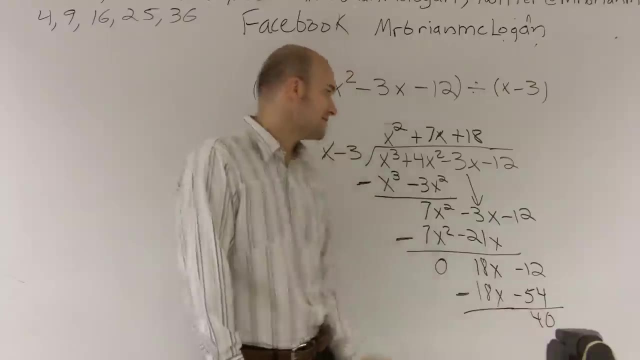 And you had to do the whole thing. now It's hard, Not even good. It's so hard is your remainder. So when I have a number at the end, that's going to be my remainder. So what this tells us is: this binomial does not evenly. 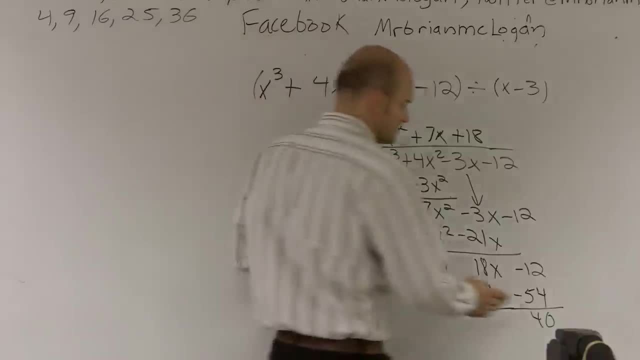 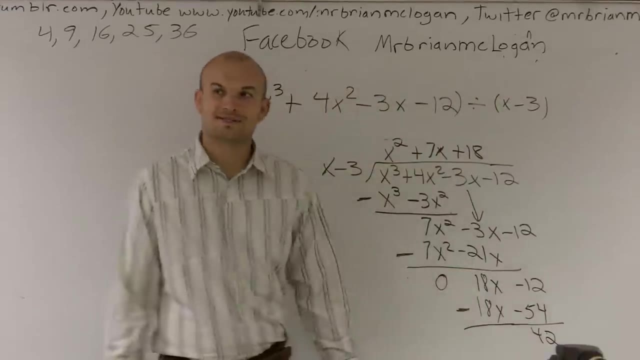 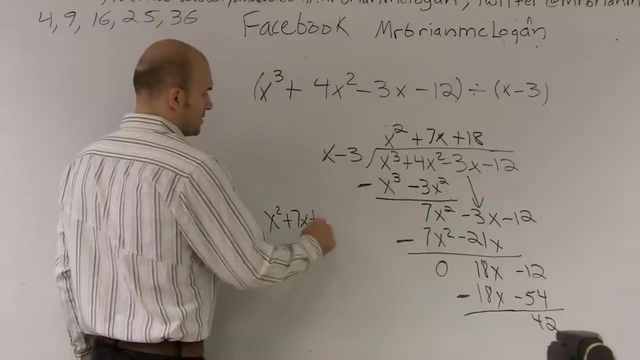 divide into this polynomial. Is it 48 and 2, right? I thought it was probably three or four times over. Thank you, So therefore my answer. this is how I write it. with the remainder, My answer is x squared plus 7x plus 18 plus whatever. 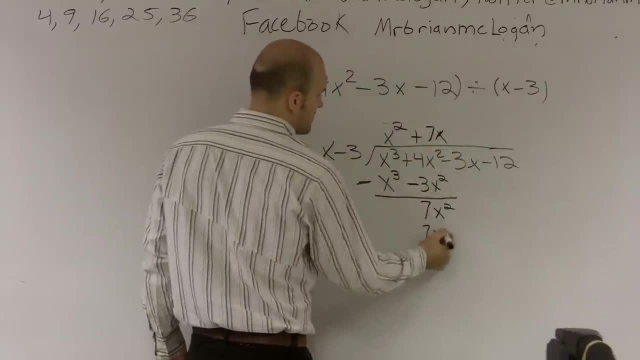 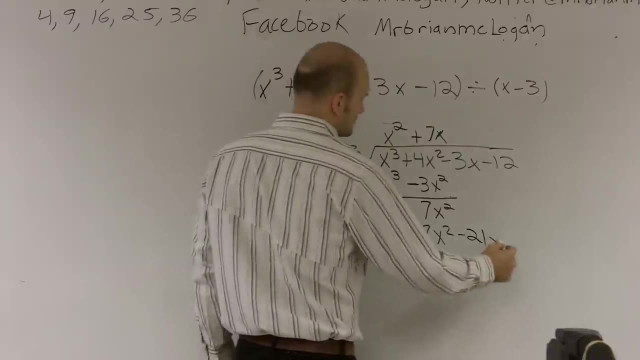 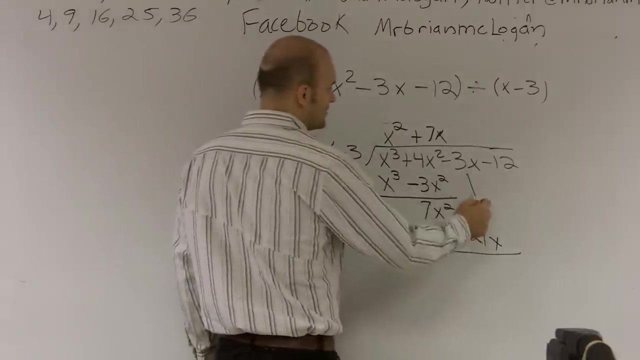 7X times X is 7X. squared 7X times negative, 3 is a negative 21X. Now I have nothing to subtract my negative 21 from right, So that's why I can bring down a negative 3X. 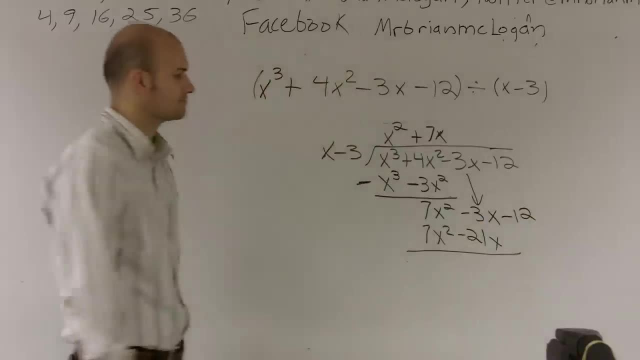 And I'll bring down the negative 12.. Just so you know, Just so. the negative 12 is not alone And this cancels out to 0.. Again, we're subtracting the whole line, right? So negative 7X squared minus 7X squared is 0.. 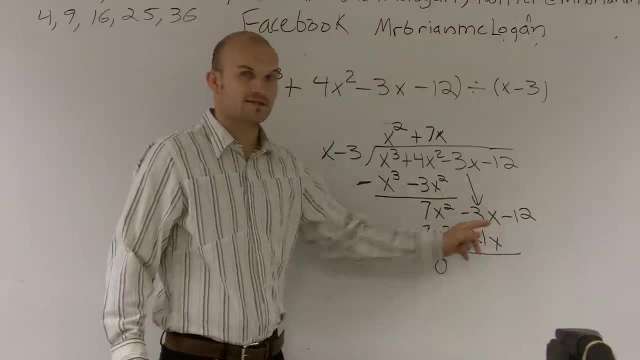 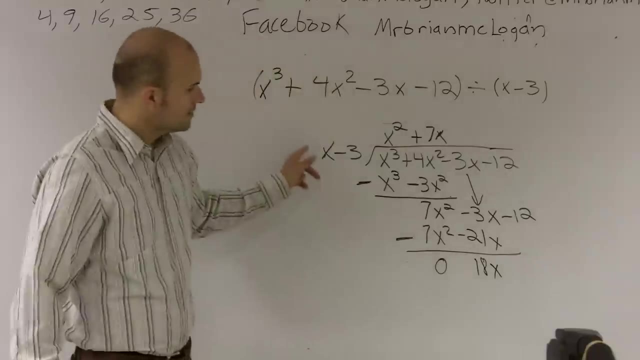 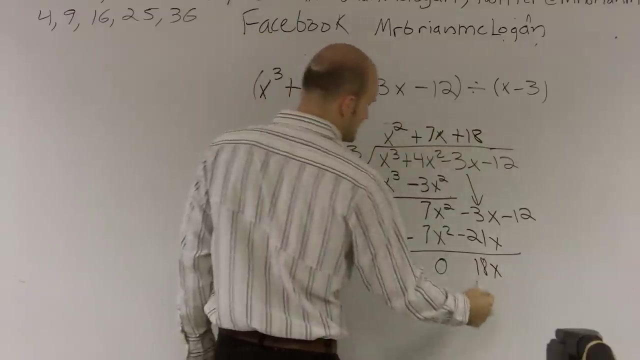 Negative 3X minus a negative 2X is going to become a positive 18X. X goes into 18X 18 times 18 times X is 18X 18 times negative. 3 is a negative 54.. 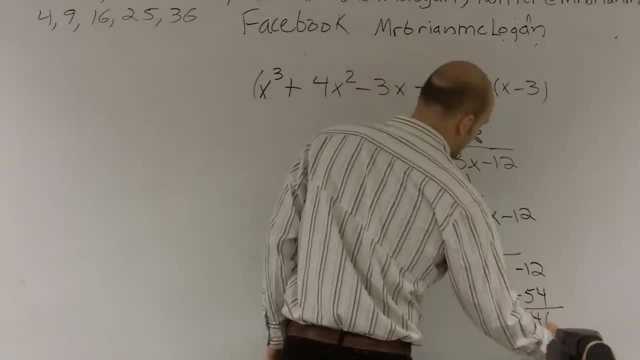 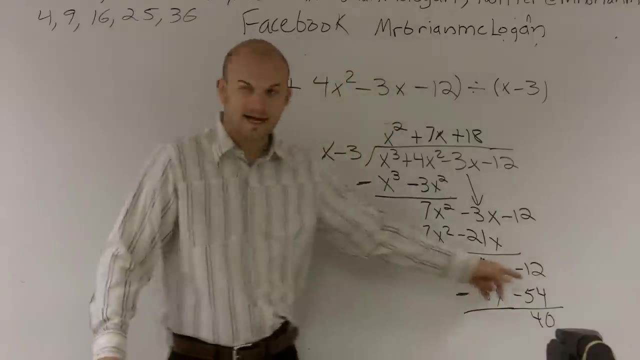 Bring down my negative 12.. This gives me 40.. Negative 12 minus a negative 54 gives me 40.. Now do you guys remember in what was it like third or fourth grade? you guys did like R When it was like 5?. 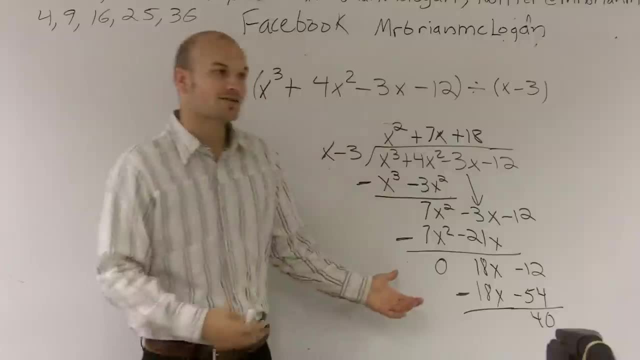 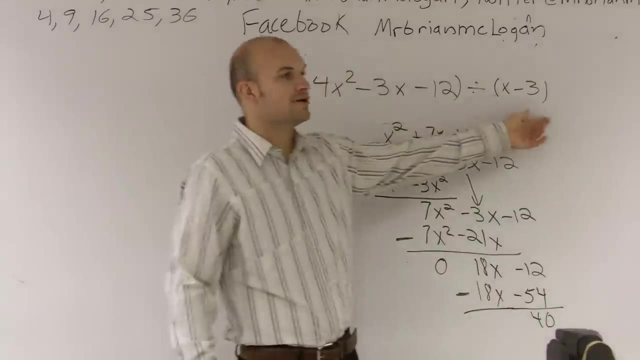 Remainder, Remainder. All right, So it was your remainder. So when I have a number at the end, that's going to be my remainder. So what this tells us is: this binomial does not evenly divide into this polynomial. Is it 48 and 2, right? 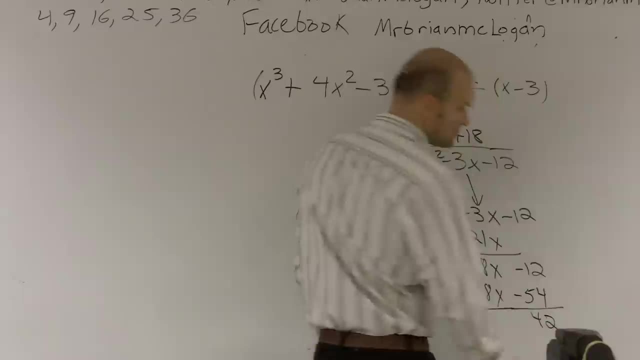 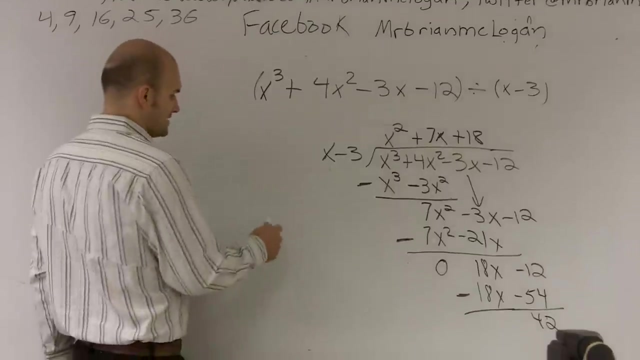 I thought it was probably like 3 or 4 times over. Thank you, So therefore, my answer. this is how I write it. with the remainder, My answer is X squared plus 7X plus 8X squared, All right. 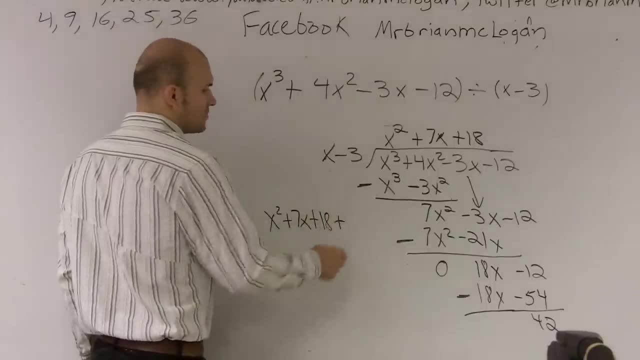 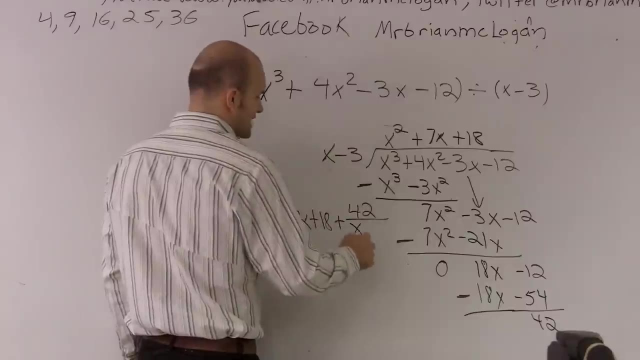 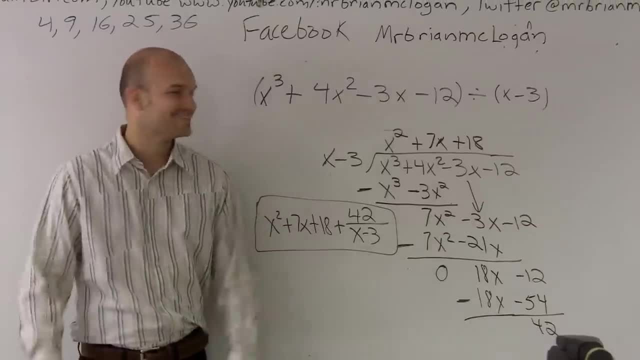 Sorry, I just messed it up, All right.